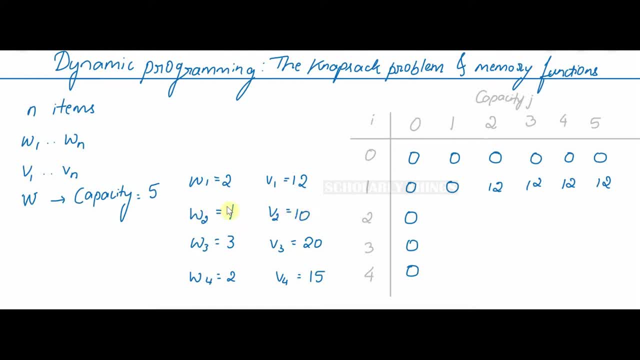 equal to 1 and value is 10.. This object can fit into the bag when the capacity is 1.. So I can write the value 10 of item 2 here. I already told that we have to consider the previous objects as well, So I 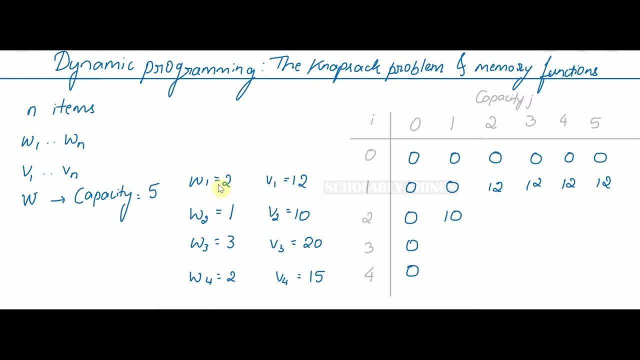 consider the first object as of now, Whichever has the maximum value. we have to take that Among item 1 and 2, though the value of item 1 is higher in this position where the capacity is 1, only item 2 can fit here. So I have written the. 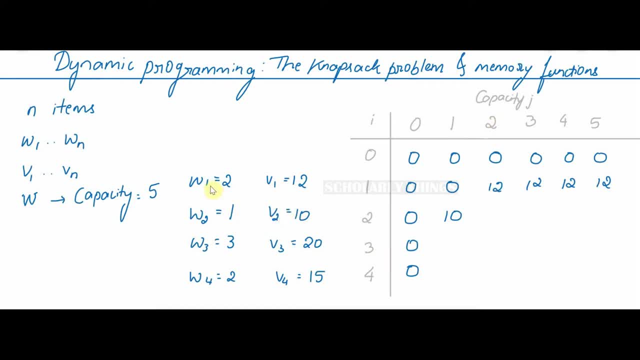 value of item 2.. That is 10.. Coming to the next value, that is when capacity is 2.. Now I need to consider both the objects. The first object, weight 2. second object has weight 1. I can fit either one of these over here. 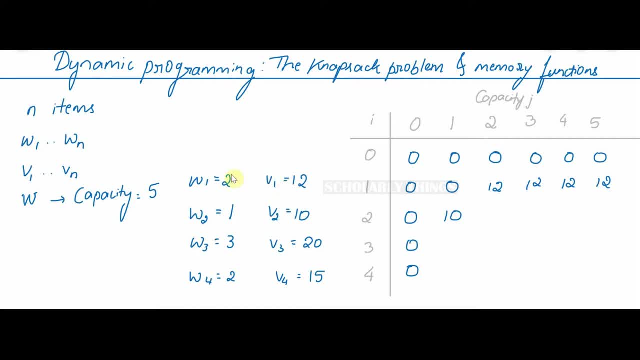 but I can see that the value of item 1 is higher, so I choose item 1. write its value over here. when the capacity of the bag is 3, I can fit both these items because W 1 plus W 2 is equal to 3. so add the values of both items and write. 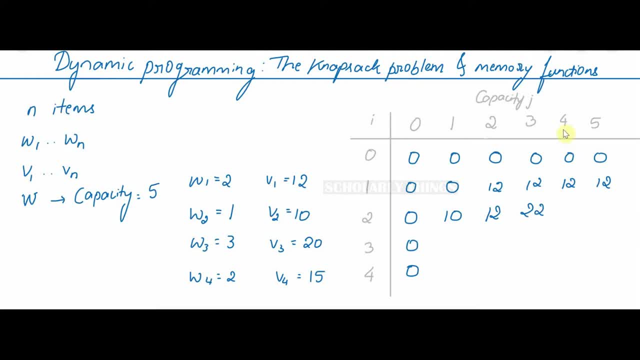 it over here. similarly, when the capacity is 4 and 5, I can fit both the items 22, 22. now let's consider the third item as well. in the capacity is 1. among these three items, I can fill only the second item. so write the value of second item 10. when the capacity is 2, I can fill the. 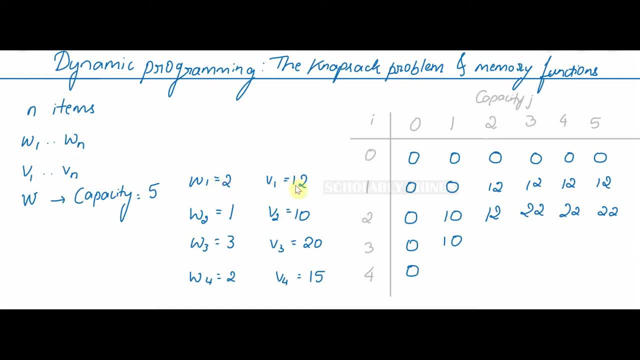 first item or the second one. the value of first one is higher, so I write that when the bag capacity is 3, I have the option of filling the third item alone or the first and the second item together. I see that if I fill first and second item, the combined value will be 22. 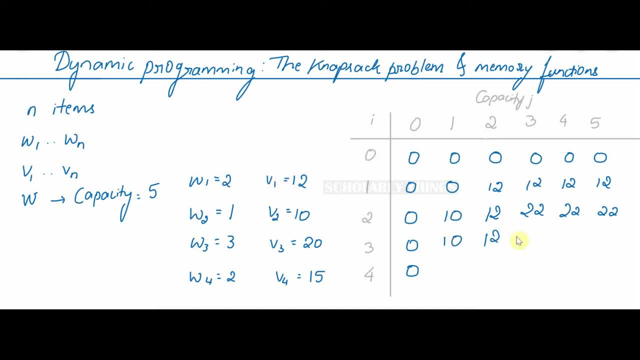 which is higher, so I can add these two items. the same process continues to fill the table as shown here. this was using dynamic programming and it is a bottom-up approach. it goes on filling the table with solutions to all smaller sub problems. some of these smaller problems or calculations are often not. 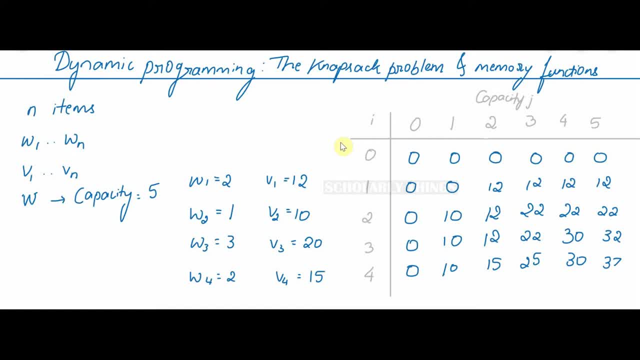 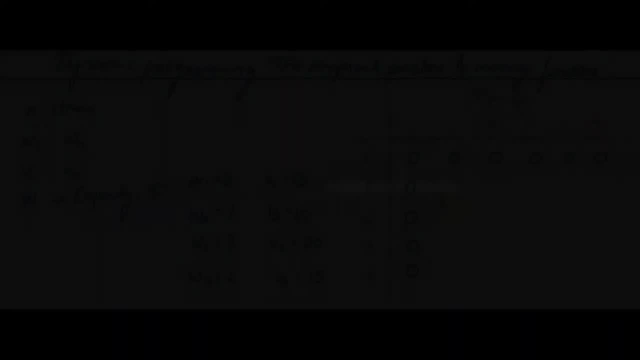 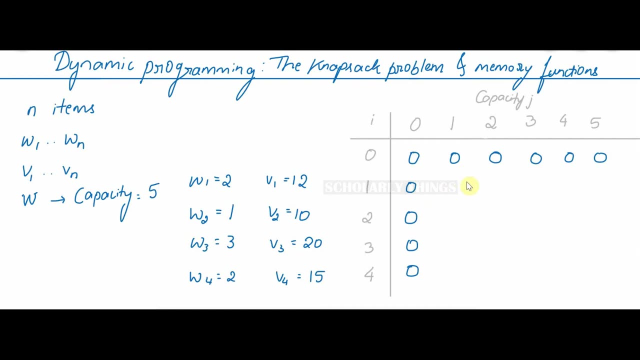 necessary. to avoid this. we need a method that would solve only the smaller problems of the table and not only the smaller problems of the table, only subproblems that are necessary, and it does so only once. Memory function method does just that: It uses top-down approach but it uses the table same as. 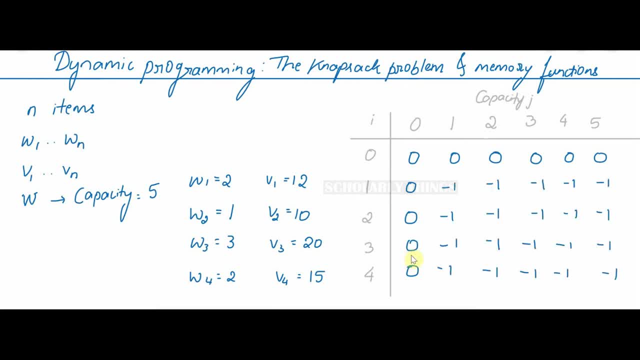 that of bottom-up approach. Initially, all entries are marked null, indicating that they haven't been calculated. While calculating, it checks the corresponding entry in the table first. If it is not null, it simply retrieves from the table. Else, it computes using the recursive call and then the result is entered in. 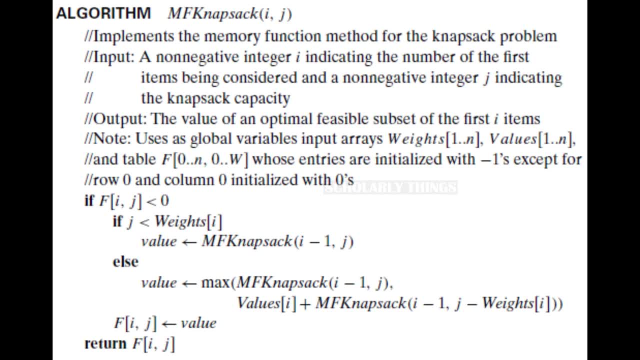 the table. This is the algorithm memory function knapsack. Let's call it MFK. If f of i- j is less than 0, then if i is less than weights of i, then value is equal to MFK of i minus 1 minus 2.. 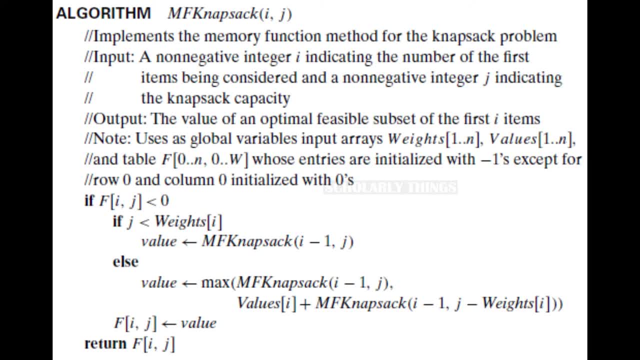 Otherwise, value is equal to maximum of MFK of i minus 1 comma j and value of i plus MFK of i minus 1 comma j, minus weights of i. Then put the value to f of i j, then return f of i- j. We need to remember these two formula. 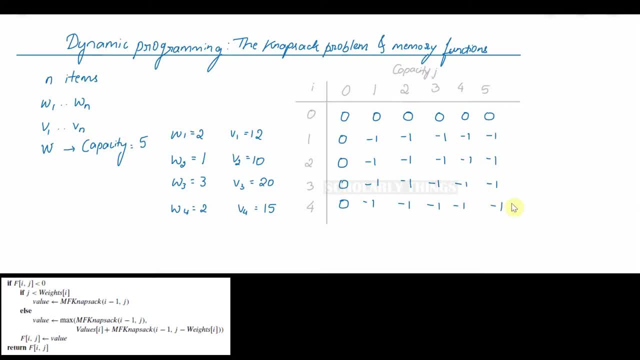 throughout our calculations We start with the last value, and the next value is the value of i minus 1 comma j. We start with the last value and then backtrack and find out solutions to only those sub problems that are necessary. Let's start with the last value, that is MFK of 4 comma 5.. Initially, all the 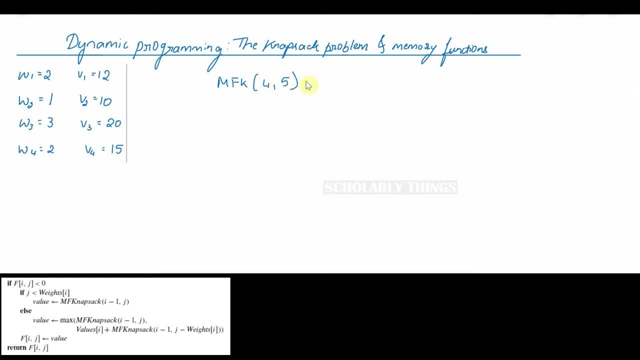 values are set to minus 1. so is this value? so f of 4 comma 5 is equal to minus 1.. The first condition is checking if this value is less than 0.. Yes, it is less. Let's check the next condition: j is less than weights. 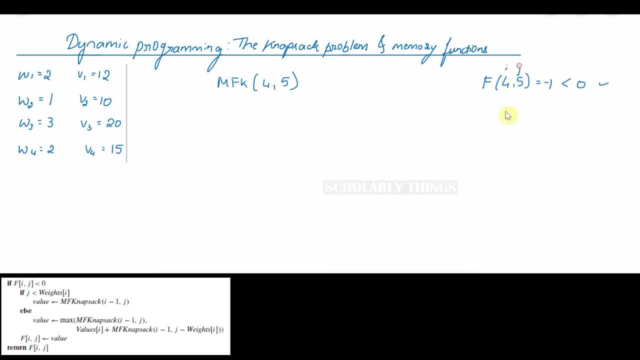 of i, This is i, this is j. So 5 less than weight of i, Weight of 4 is 2.. 5 less than 2 is wrong, So we perform the else part. Value will be maximum of MFK of i. 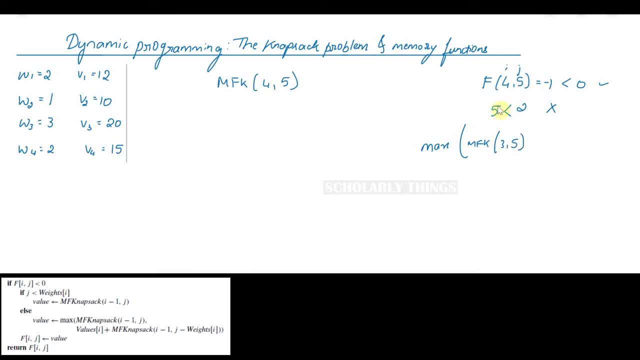 3, 5, i-1 is 3, j is 5, value of i is 15 plus mfk of i-1 is 3, j-weight of i, that is, 5-weight of i, is 2.. It will be max of mfk of 3, 5, 15 plus mfk of 3, 3.. So we will be taking the maximum value. 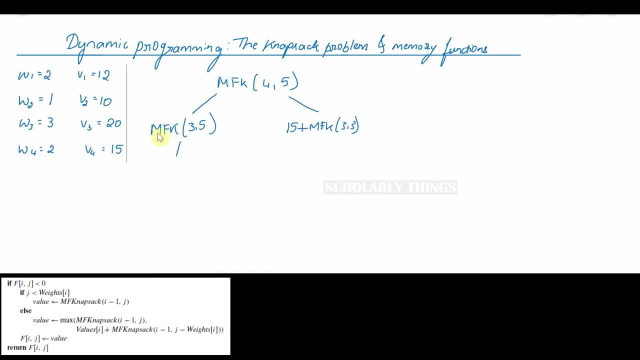 among these two. Now let's take mfk of 3, 5.. The algorithm is recursively called mfk of 3.. So this time it is f of 3, 5.. The value is minus 1 initially, which is less than. 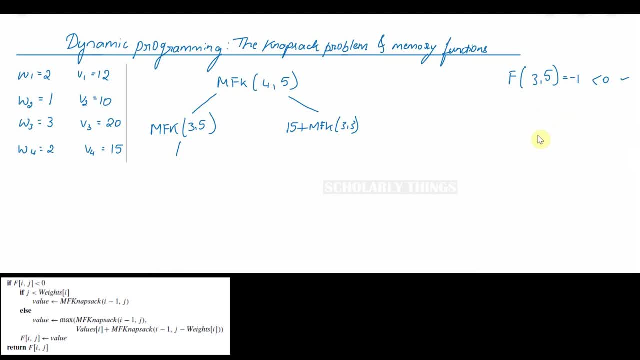 0, correct. Then check if j is less than weight 5 less than weight of 3 is 3,. 5 less than 3, wrong. So value will be max of mfk of 3.. 2,, 5, the value of i is 20 plus mfk of i-1, that is 2, j-weight of i, 5-weight of i is 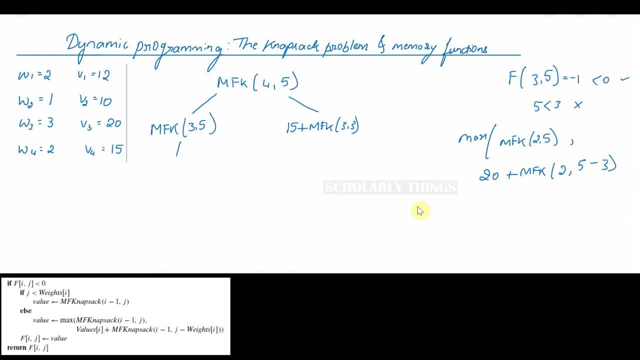 3.. It will be max of mfk of 5,, j-weight of i is 3, j-weight of i is 3,, j-weight of i is 3.. So we will be taking the maximum value of mfk of 2,, 5, 20 plus mfk of 2, 2.. So for 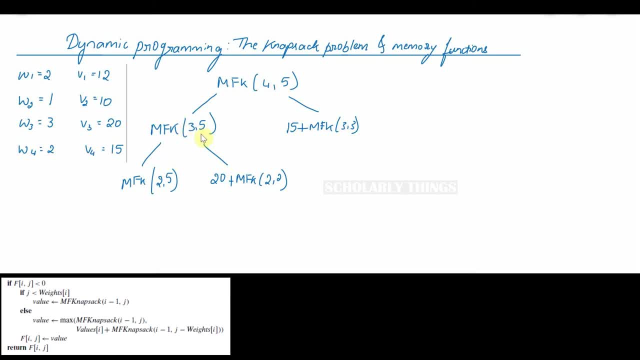 finding out the value for mfk of 3, 5,. we need to find the maximum among these two values and assign it to mfk of 3, 5.. The algorithm calls itself recursively, as shown here. We need to find out all these values: mfk of 1, 5,, mfk of 1, 4 plus 10, all. 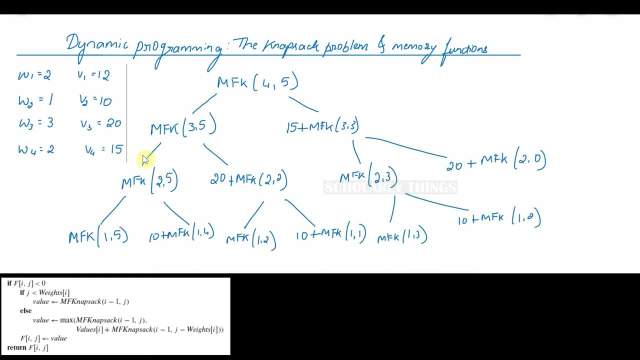 these and then go on finding the maximum among the two values till we reach the final point. I'll show for one value: mfk of 1, 5.. We'll be considering the second case. This will be max of mfk of 0, 5.. 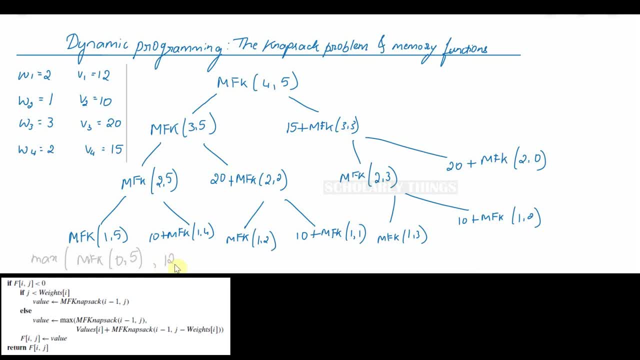 5 comma 12, plus MFK of 0 comma 5 minus 2 MFK of 0 comma 3. as we saw in the table when the weight was 0, it is 0. so 12 plus 0 is 12 maximum among 0 and 12. 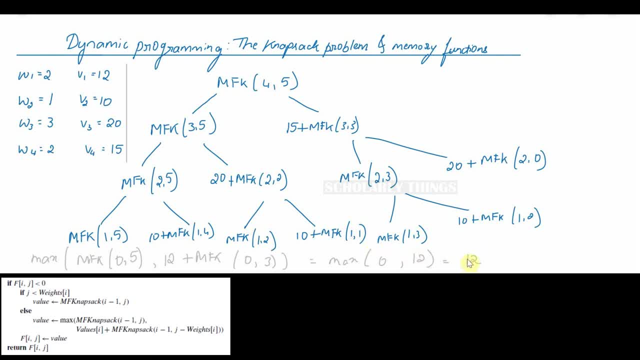 is 12. so therefore, MFK of 1 comma 5 is 12. similarly, we find out MFK of 1 comma 4 to be 12. 10 plus 12 is 22. MFK of 1 comma 2 is 12. MFK of 1 comma 1 was found out to be 0. 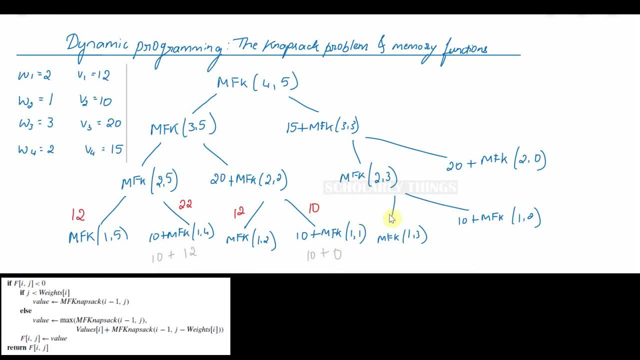 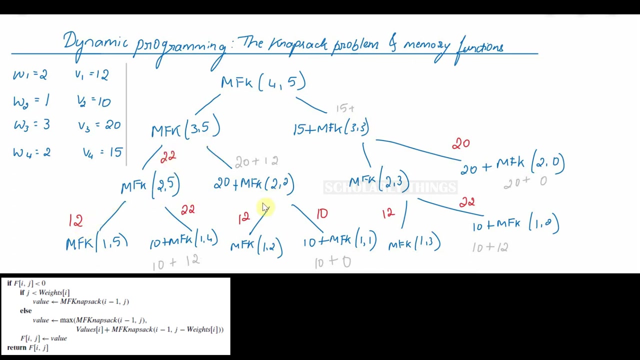 10 plus 0 is 10. ok, MFK is 12.. MFK is 12.. 10 plus 12 is 22.. MFK is 0.. 20 plus 0 is 20.. Here, maximum of 12 and 22 will be 22.. Maximum of 12 and 10 will be 12.. This value becomes 20 plus 12, that is, 32..